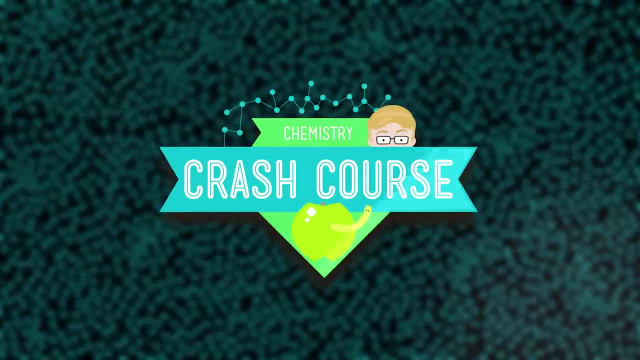 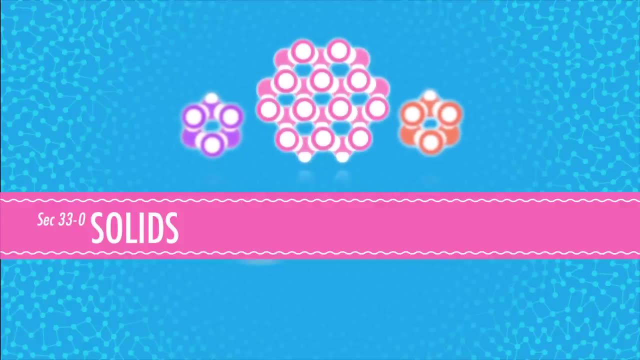 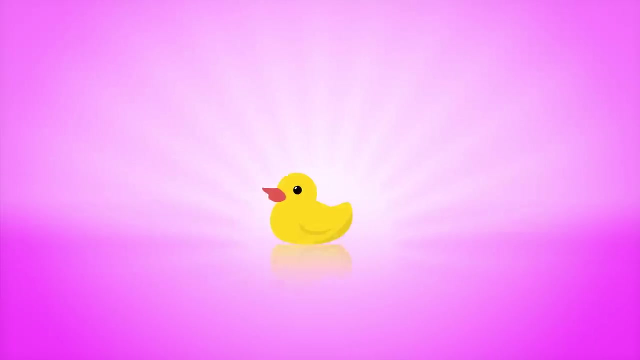 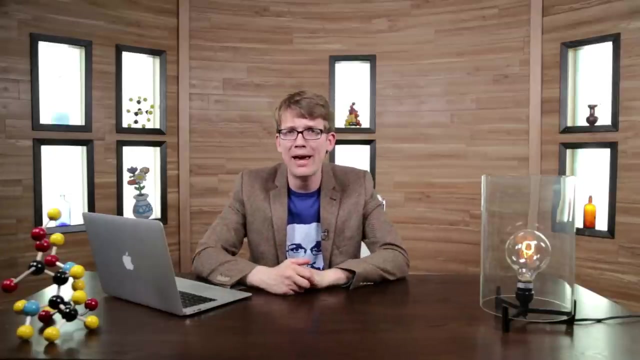 what chemicals really are. The category of amorphous solids includes things that you might expect like foams and gels, and colloids like mayonnaise, rubber waxes and some biological tissues such as fat. They also include some things that you might not expect like coal, the thin silicon panels. 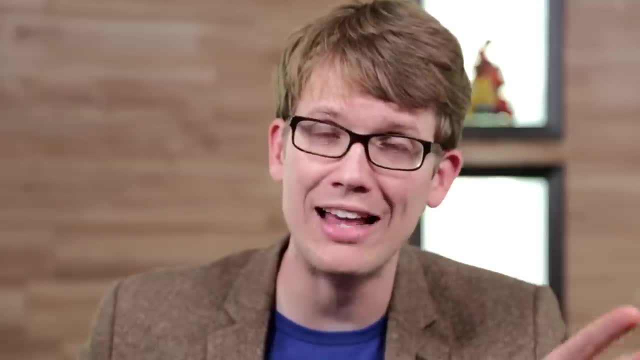 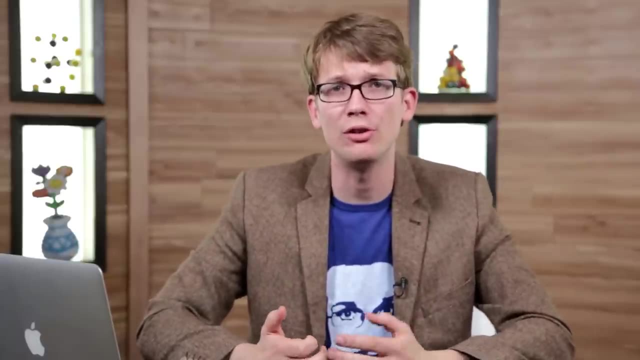 used in semiconductors and even glass. That's right. despite what you may have heard, glass is not a liquid. I don't know who made that up In chemistry. amorphous doesn't mean soft or even flexible, although many amorphous 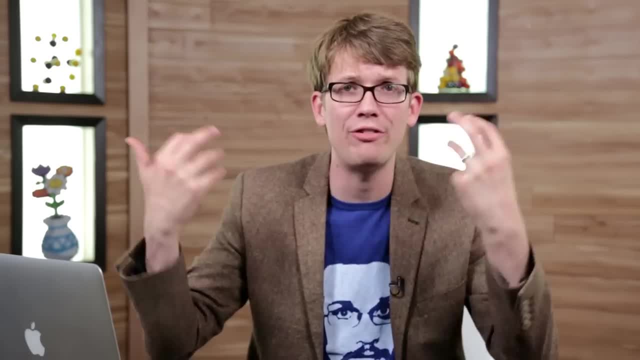 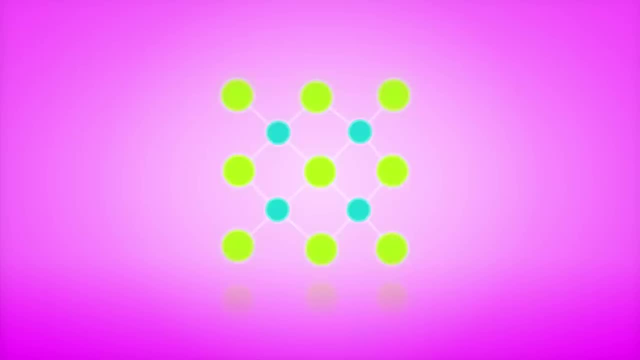 solids are both of those things. Instead, the classification is all about the fact that their atomic structure is disordered or random. Amorphous solids do, however, have a couple of macroscopic properties in common. First, it is important to understand that, because the particles in an amorphous solid 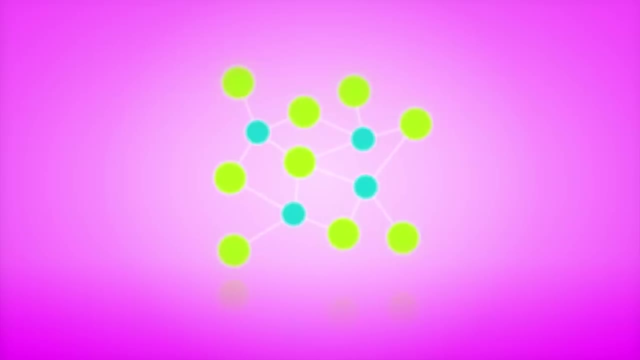 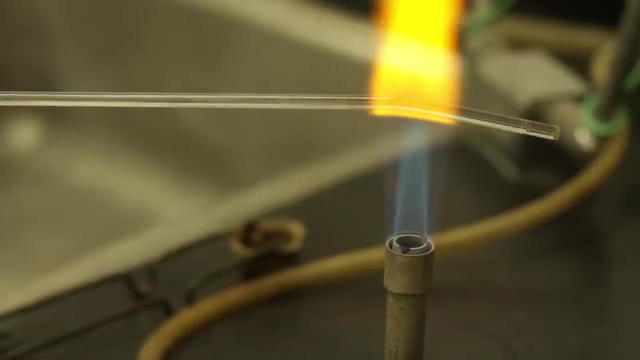 are arranged randomly, the strengths of the bonds holding them together are also random. That's what causes amorphous solids to melt gradually, like this glass tube. As the material is heated, the weaker intermolecular bonds break first, then the stronger ones break. 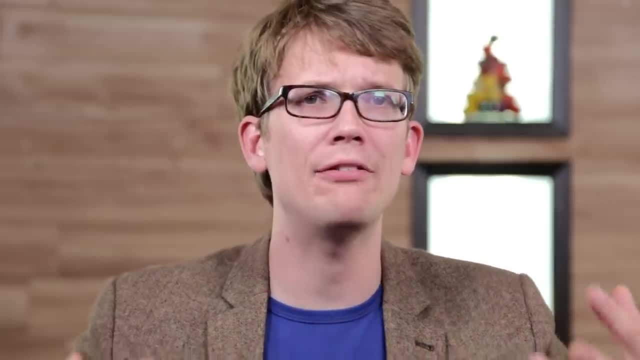 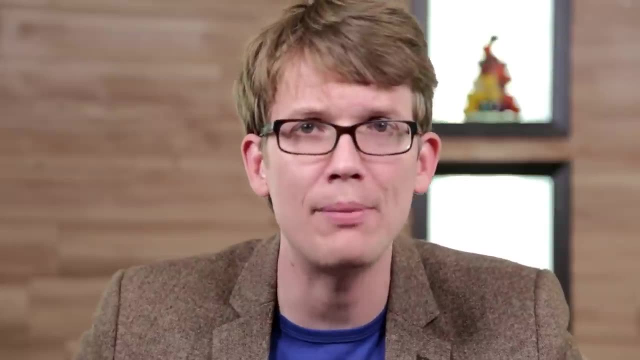 as the energy threshold is broken by heat. So amorphous solids don't have the sharp, discrete melting points of things like ice, which melts exactly at zero. Instead, they melt over a range of temperatures as the heat energy increases. Amorphous solids also respond to stress very differently than crystalline solids, Because 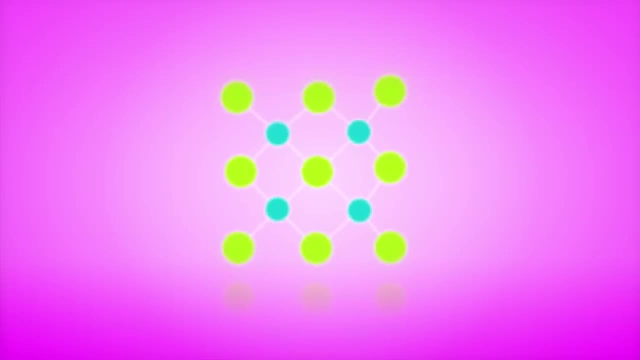 the arrangement of crystalline solids is so orderly they're often very easy to break along a plane that falls between adjacent molecules, And when they break they tend to do it along straight lines. the way cutting a diamond creates perfectly smooth facets, But with many amorphous solids it's hard to find a plane like that, No matter how you. 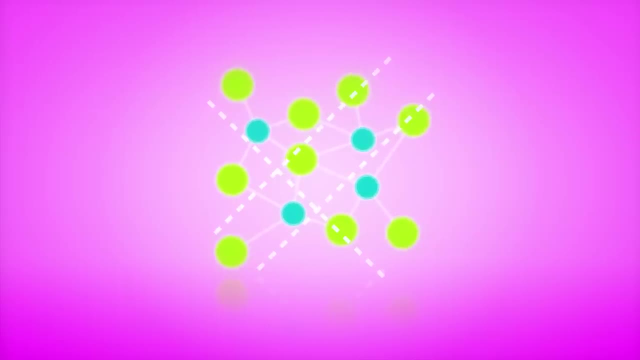 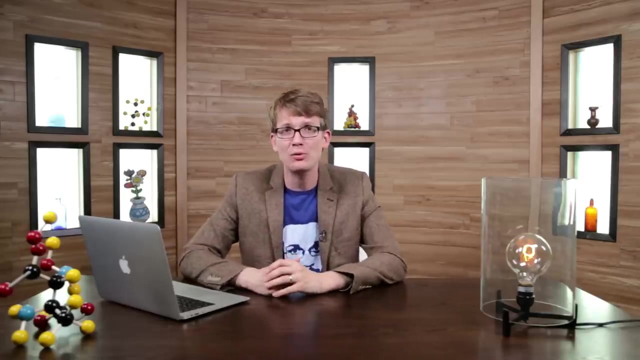 attack it, you'll usually run into molecules that are sitting right in the middle of that plane resisting the break. And even hard amorphous solids that do break under pressure rarely do it along straight lines. That's why broken glass ends up in crazy random shapes and why coal looks like 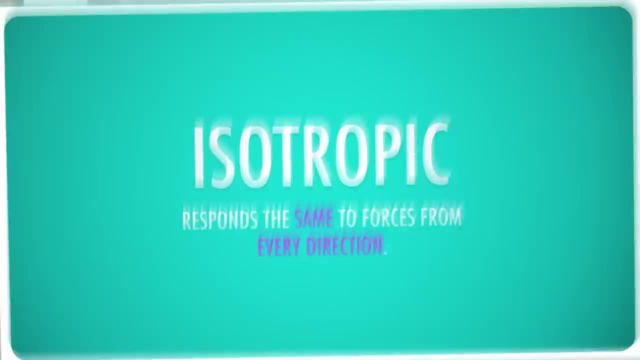 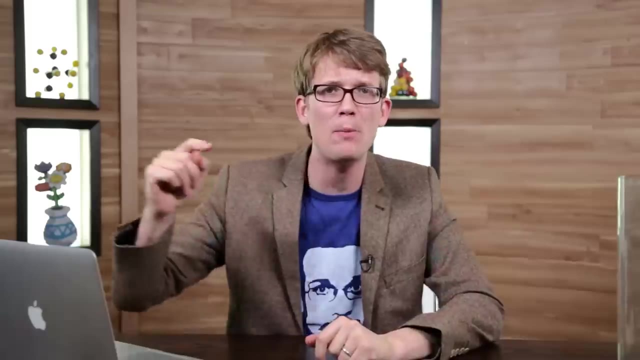 a random rock, not like a nice, orderly crystal. We have a name for this: Amorphous solids are isotropic, meaning that they respond to stress in the same way in every direction, No matter which direction you poke a piece of clay or hit a piece of. 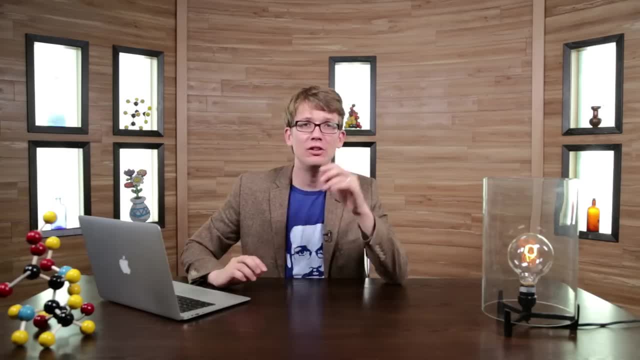 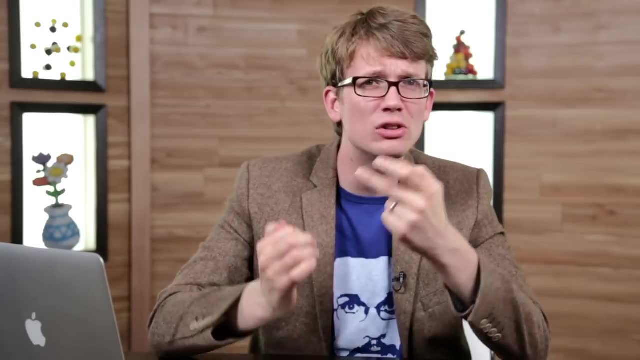 glass. its resistance to breakage will always be similar, But crystalline solids are anisotropic. They break differently depending on which plane you hit. Speaking of diamonds, you probably think of crystalline as things that look sort of like that, But there are actually three different types of crystalline solids and they cover. 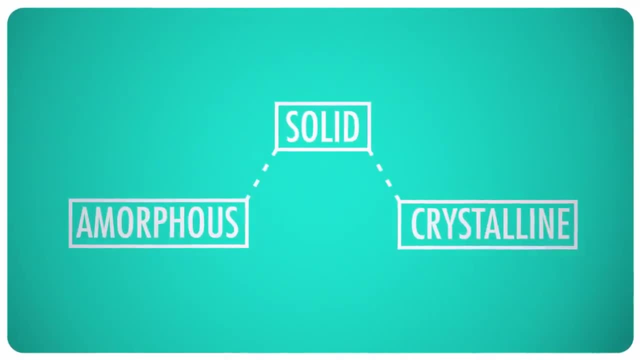 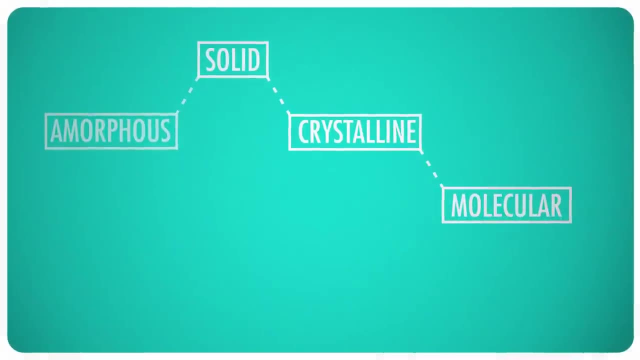 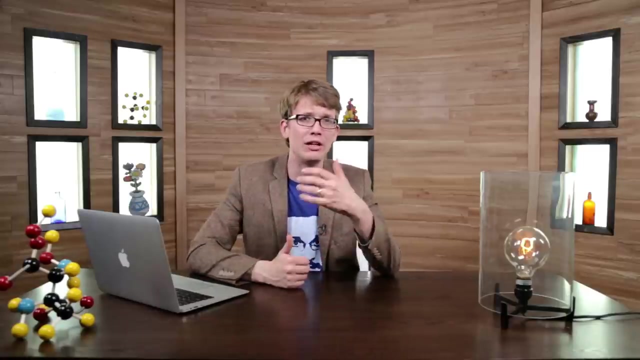 a huge array of materials, some of them pretty surprising. Those types are based on composition. They can be molecular, ionic or atomic. Molecular solids are made up of covalent compounds that form an orderly crystalline structure as they solidify, while their molecules remain unchanged. Examples include things like water. 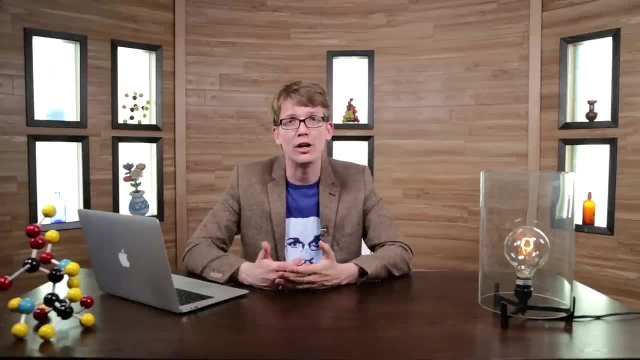 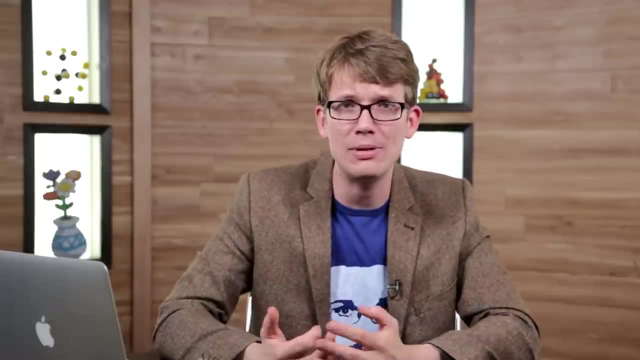 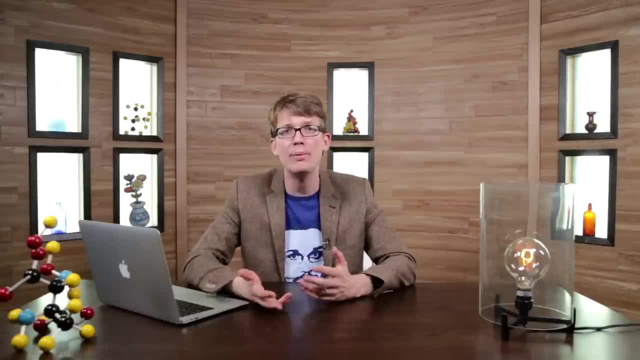 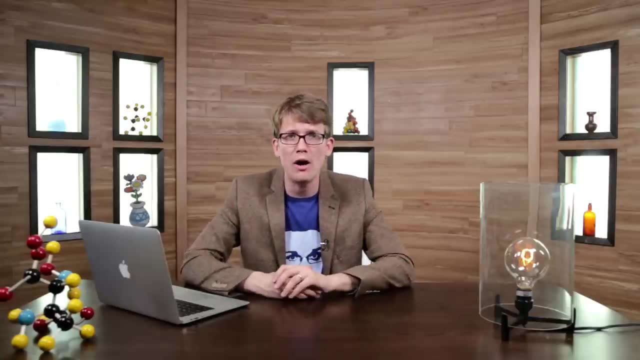 Ionic solids are basically the solid forms of things we think of as ionic compounds Like sodium chloride or table salt, calcium carbonate, which is chalk and limestone, and magnesium sulfate, otherwise known as Epsom salt Because they're made of ions. they're often soluble in water and other polar solvents. 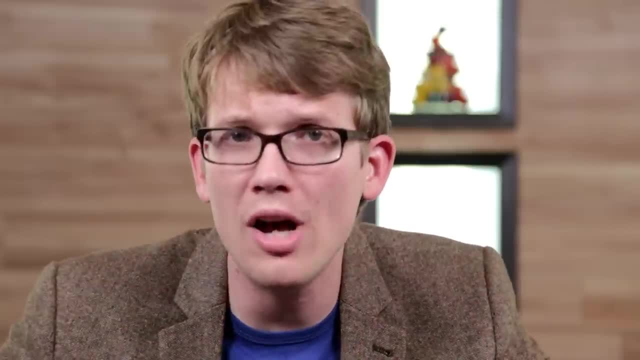 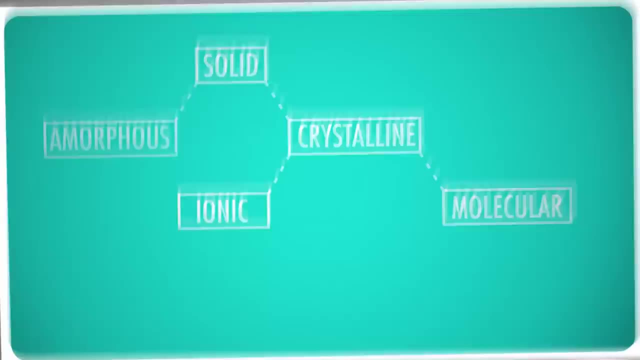 but they have very high melting points. So table salt would be gone in no time if I put it in water, but if I applied heat directly to it it wouldn't melt until the temperature reached 801 degrees Celsius. Atomic solids, as the name suggests, are made up of individual atoms, not molecules at all. 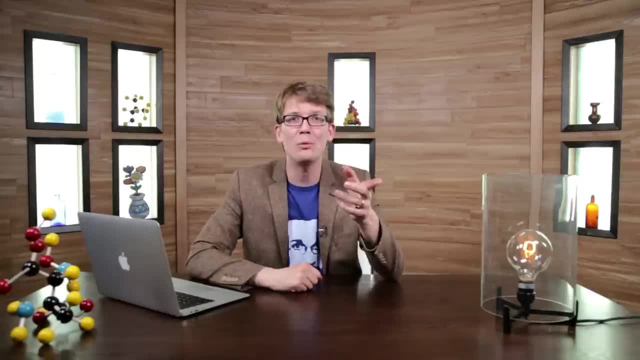 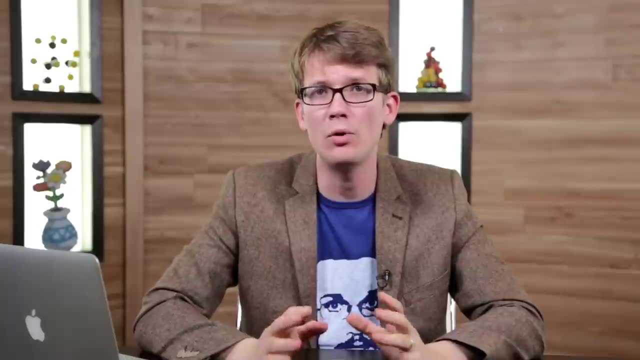 Well, there are actually three types of atomic solids too: Network solids, group 18 solids and metals. Network solids are so interesting and important that we're going to cover them in a separate lesson. I won't get into it now, except to say that the atoms basically form a rigid crystal structure. 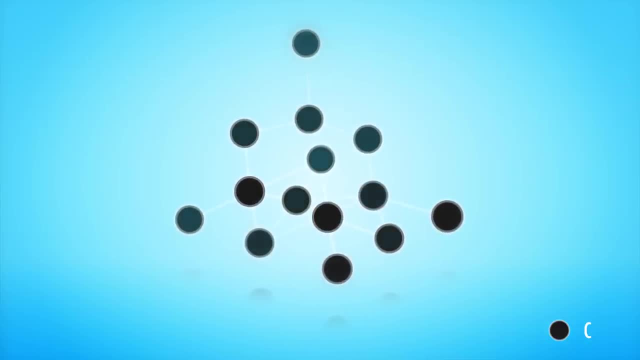 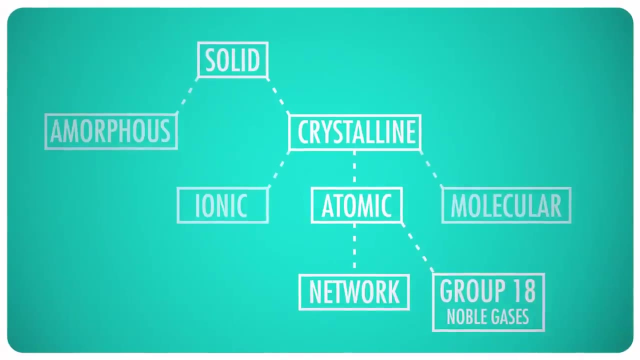 A diamond, for example, is just a big crystal made of carbon atoms, so you can think of diamonds and other network solids as really giant molecules. Group 18 solids, meanwhile, are the solid-phase materials of the noble gases. group 18 on. 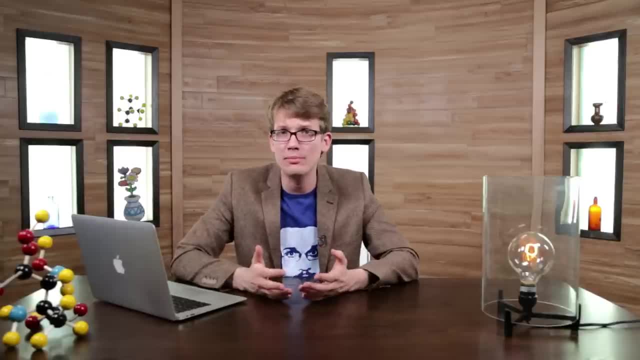 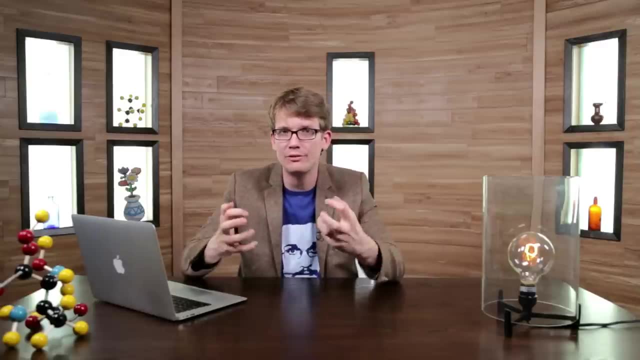 the periodic table. Sometimes noble gases have a little interest in interacting Even among themselves. it's very hard to cool and pressurize them enough to make them form a liquid, and even more so to make them solidify. So when they do crystallize, the atoms are held together by weak little van der Waals. 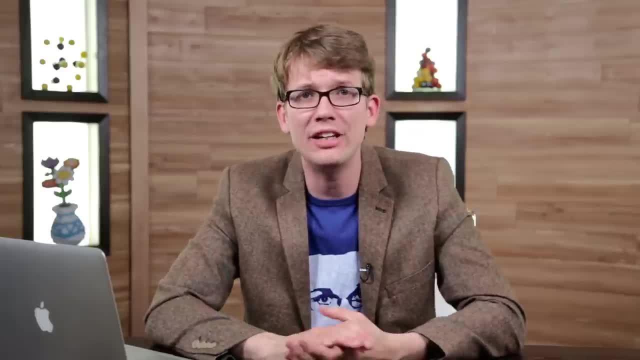 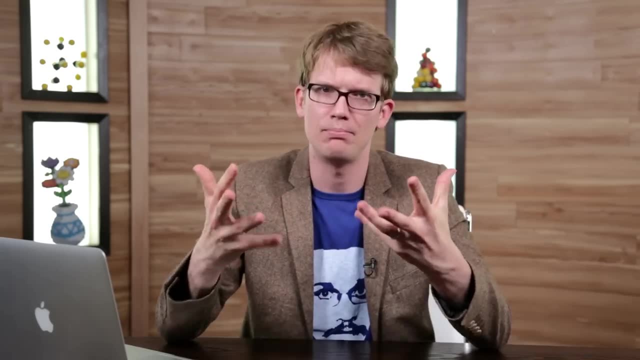 forces not stable at all, to say the least, so they don't tend to stick around for long. Because of this, they're really rare and not something that you'll like ever encounter, unless you go on to study them specifically. 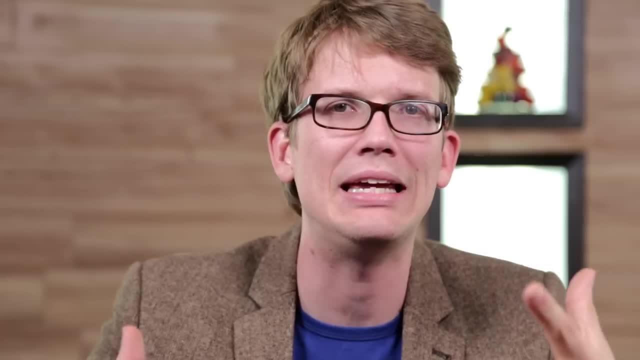 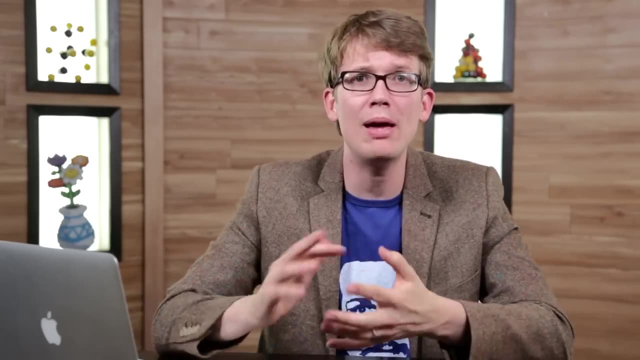 But metals, You know metals, They're everywhere. You're probably looking at me On a device made of metals. You probably have metal in your pocket. You might have metal in your teeth And, yeah, you probably don't think of metals as crystals. but remember, the key is that 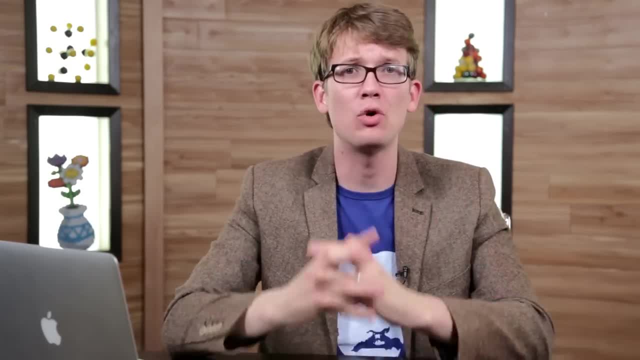 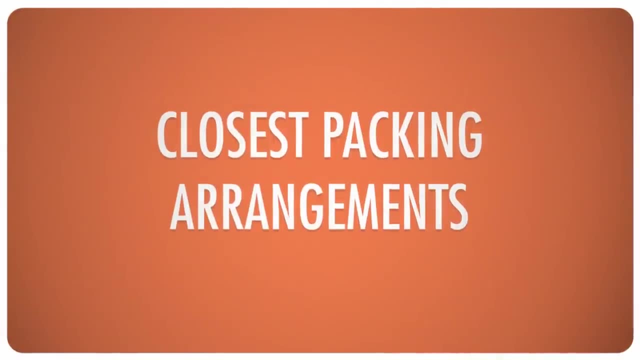 their atoms are arranged in an orderly way. The atoms in fact form several different arrangements in order to best take advantage of the space in the structure. These structures are called closest packing arrangements. To picture how it works, think of metal atoms as spheres and consider how they can pack. 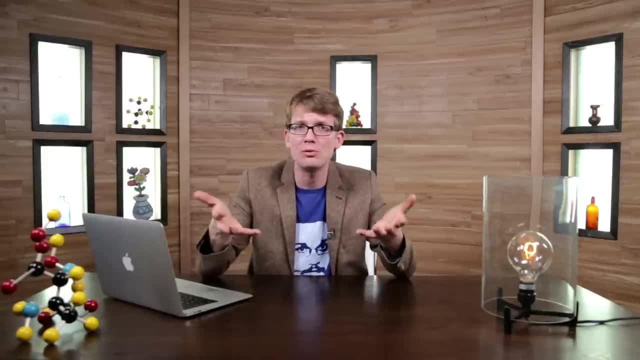 together in the most efficient way as possible, Like: imagine if you have to fill a box with as many ping pong balls as you can. The atoms stack just like the ping pong balls would. 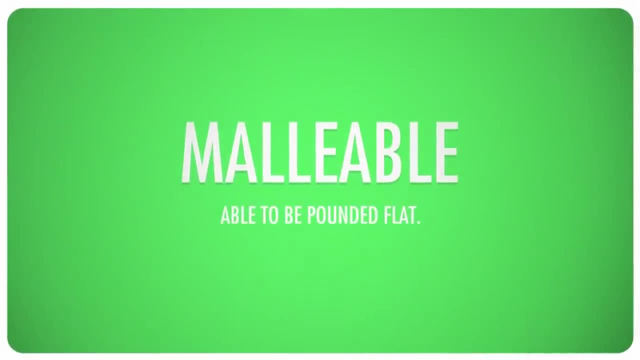 is what we would have to think of as light metals, though Most metals are quite malleable, meaning that they can be pounded into various shapes, and ductile, meaning that they can be stretched out into wires. 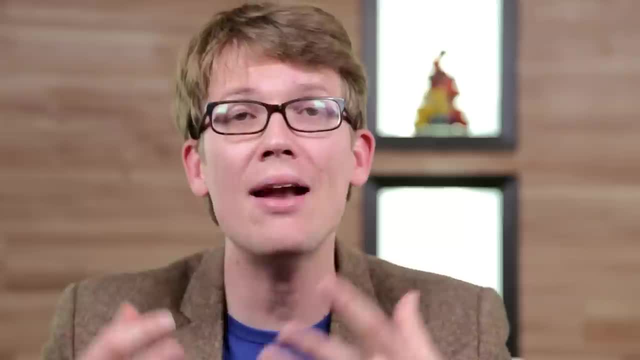 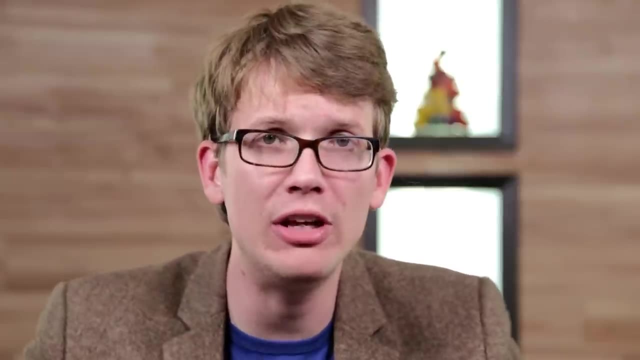 Both of these characteristics result from the nature of their atoms and the bonds between them. The atoms in metals are large, so large that the valence electrons aren't held very strongly by the nucleus. This gives them much more freedom to move around than electrons on most elements. 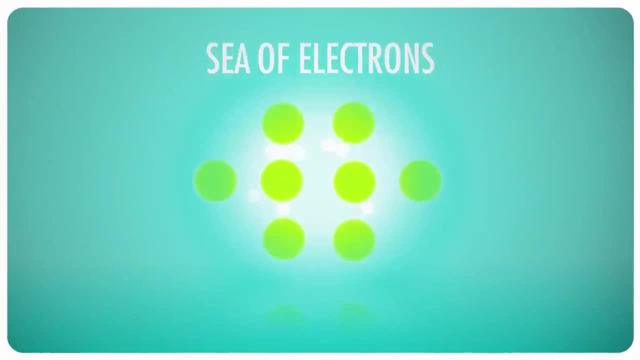 So instead of belonging to a single atom, they form a kind of sea of electrons, wandering from one nucleus to another. These freely moving electrons are in fact, the main reason that metals can conduct a heat and electricity so easily. It's actually more accurate to say that the electrons form large, somewhat unstable orbitals. 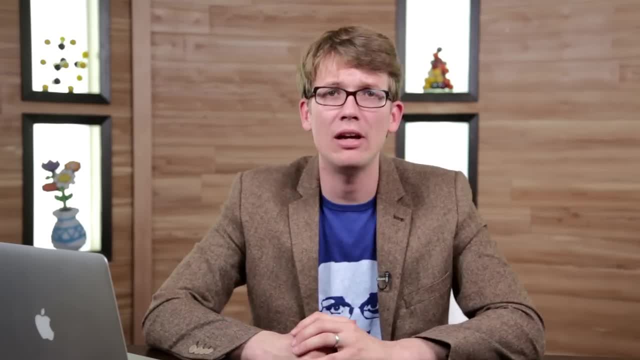 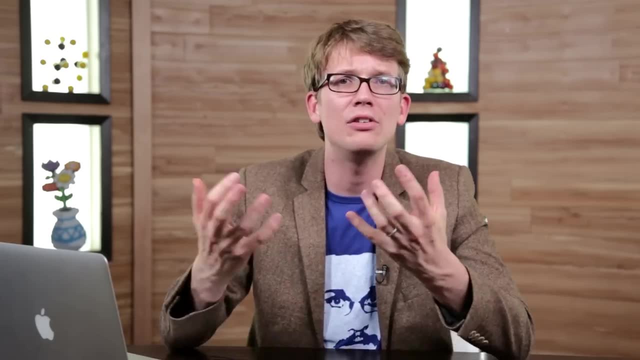 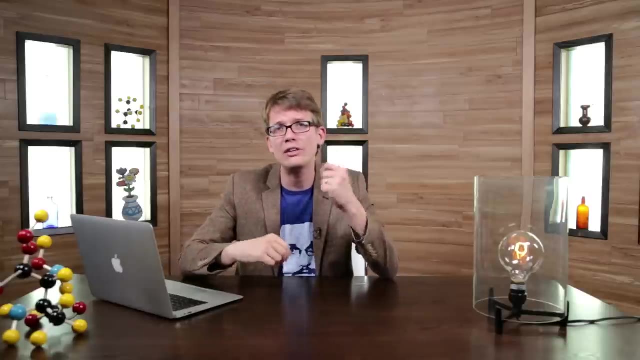 around collections of atoms. The nuclei are tightly bonded together by the electrons that are all around them, making the metal structure extremely strong, But the bonds are uniquely flexible, allowing the kinds of deformations that we're accustomed to from metals. Despite the crazy array of solids that classify as crystalline, they do all have certain things. 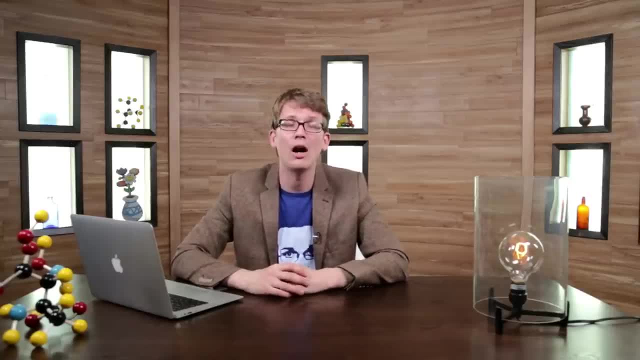 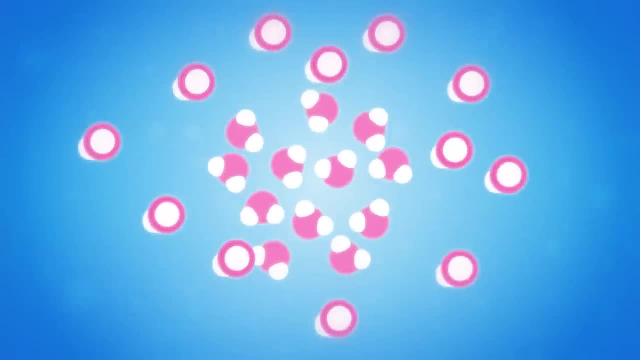 in common And, as usual, most of their common characteristics are related to their bonds. Since all the bonds in a crystal are the same length, they're all equally strong, which means they can be broken by the same amount of energy and their melting points. 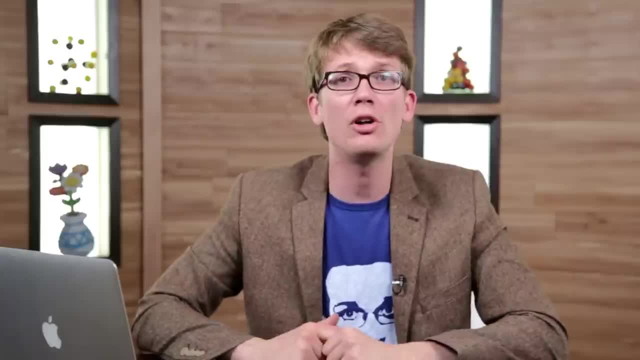 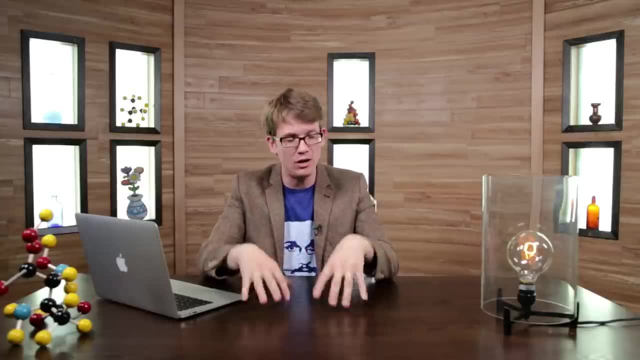 are very specific temperatures, not broad ranges. Crystalline solids are also generally more brittle than amorphous ones and, as I mentioned, respond to force differently in different directions. It's kind of crazy to think that all of the different things that we think of as solids